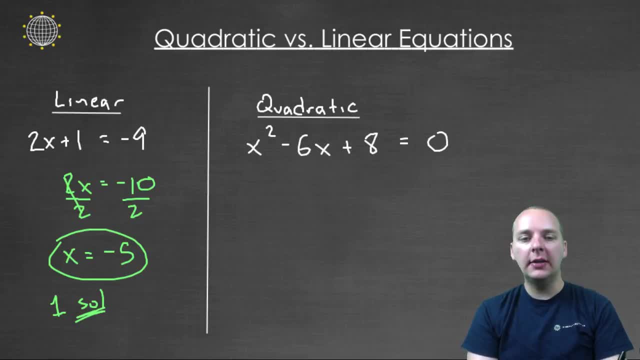 equation. Well, you see, if you try to solve for x, Let's say you try to maybe isolate this x the same way, Subtract the 8 and subtract the x squared, and divide by negative 6, and do all those sorts of things, Your x is actually going to be in terms of x squared, because you would. 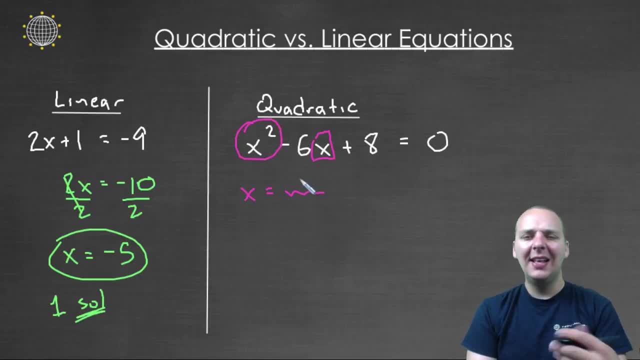 have to put the x squared on the opposite side from x, And that just doesn't make any sense. You're not going to get a numerical answer for x that way. So the approach is dramatically different, Because you have x's and x squared's- these aren't like terms, and so you can't just isolate. 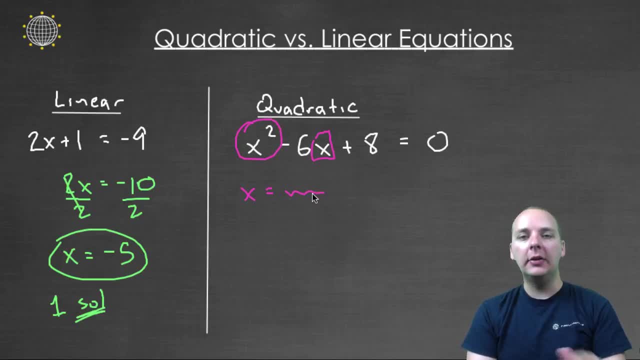 a single one of these guys. So we're going to have to have dramatically different approaches and there are a couple different ways you can do this. But to solve this type of equation, I just want to emphasize the fact that it's very different than solving a linear equation. 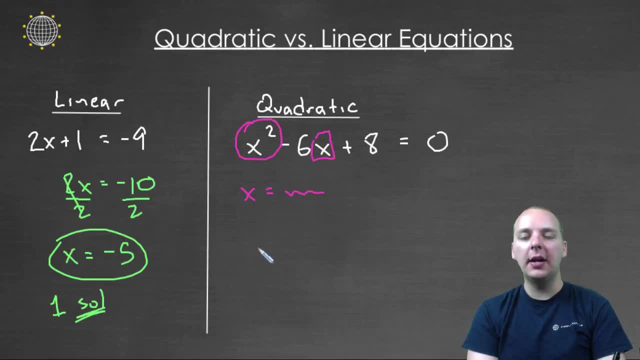 And not only that. let's actually look at what some of these answers would be, And I'm not going to go through how I got these answers. The answers for this one would be 2 and 4. Meaning, if you plug in a 2, it will make the. 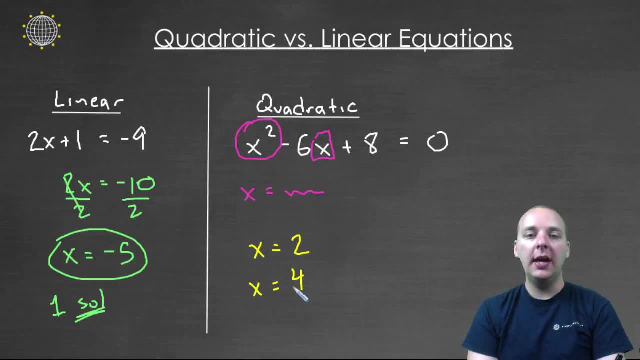 left side equal 0 and make the equation true. And if you plug in 4, it will also make the equation true. So this guy in fact has two solutions, Which is kind of interesting. Now, why is that? Why do linear equations only have one and quadratic equations sometimes? 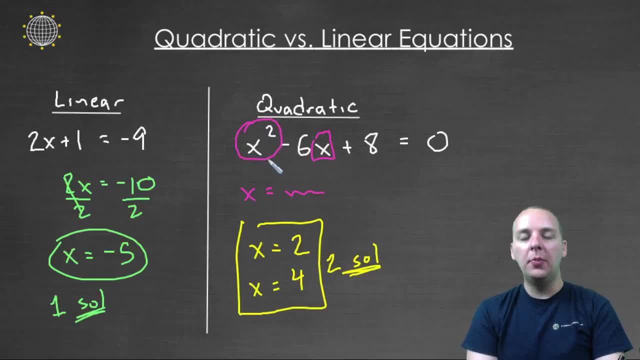 have two. They don't always have two solutions, But in this case it does. It's because of the square term right here. It's because of the square term right here. It's because of the square term right here, And so we just have a lot of differences between quadratics. 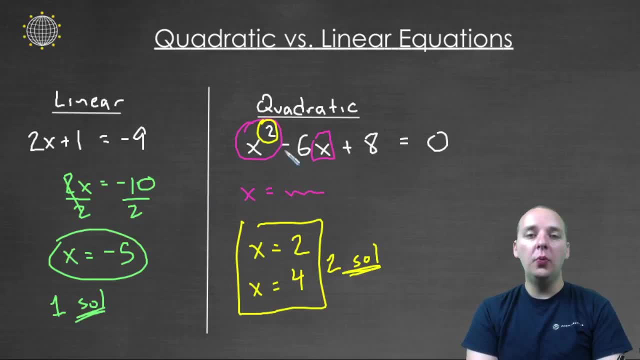 and the linear equations that we're comfortable with. Now, what will be the approach for solving quadratic equations? Again, I'm not going to get into a lot of those details, And there are a few different techniques to solve quadratic equations, But one of the techniques uses: 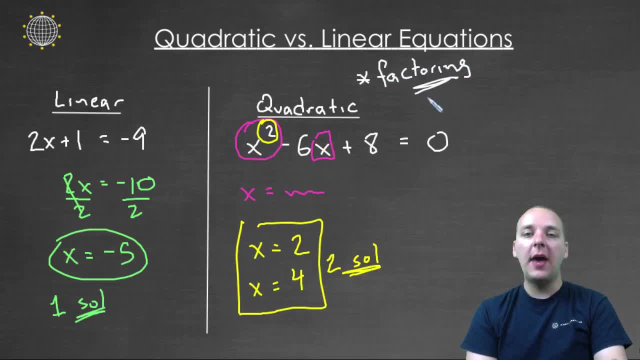 factoring, And that's why we've been studying factoring so hard. over the last few videos, It's been in anticipation that we're going to be able to solve quadratic equations, And so we're going to be able to solve quadratic equations, And so we're going to be able to.